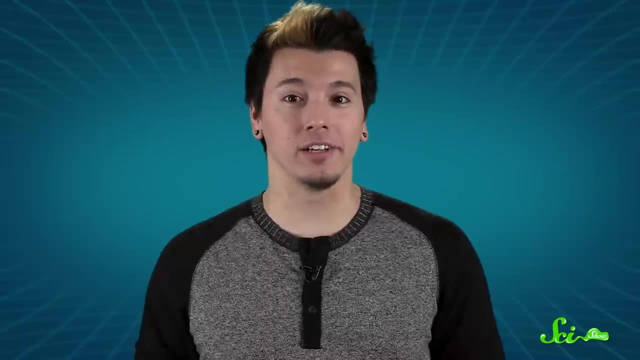 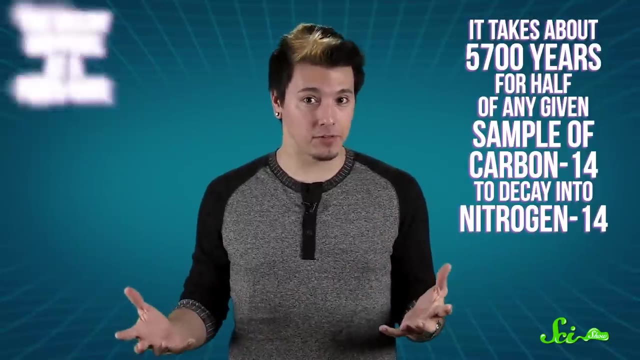 And luckily for scientists who specialize in studying old biological material, like archaeologists, this decay process happens at a fixed rate. We know that it takes about 5700 years for half of any given sample of carbon-14 to decay into nitrogen-14.. 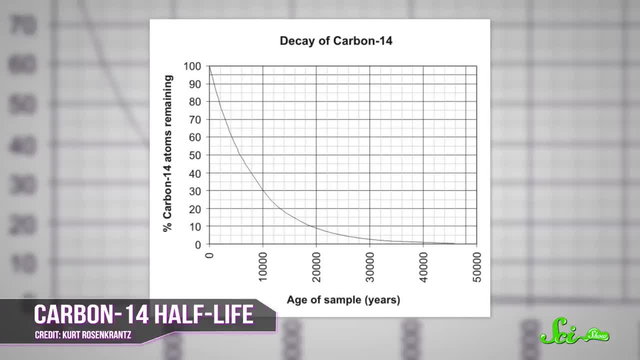 This time span is known as its half-life. So after one half-life you'll have half of the C-14 that you started with. After two half-lives you'll have one quarter, After three you'll have an eighth, and so on. 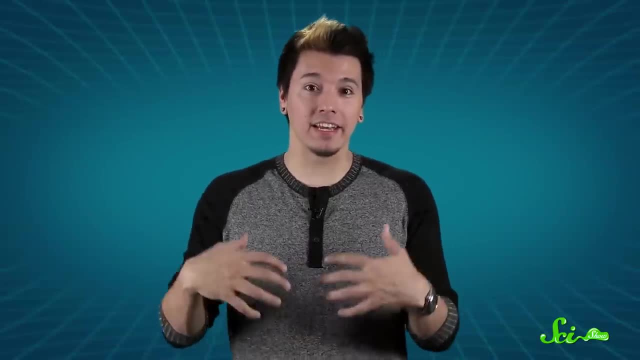 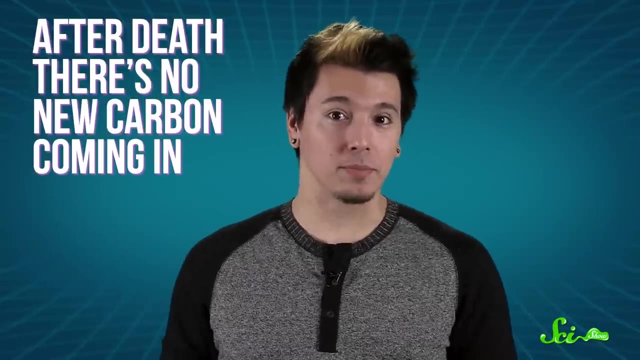 This is useful for dating dead stuff, because while living things are constantly taking in carbon about as fast as it decays inside them, after death there's no new carbon coming in. So when the C-14 decays inside the dead organism, the proportion decreases. 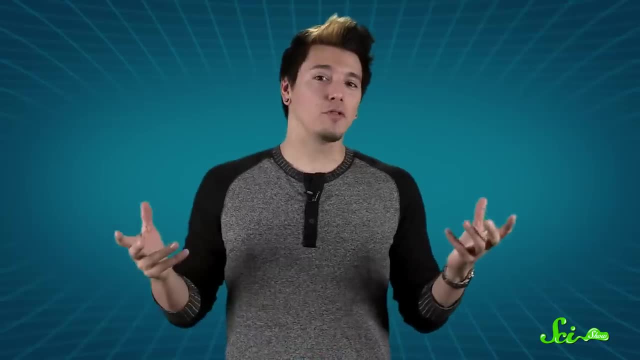 More importantly, it decreases at the same rate, No matter what the dead thing is. So let's say you find an old piece of a dead tree, Since we know that about a trillionth of the carbon atoms living in the thing are carbon-14,. 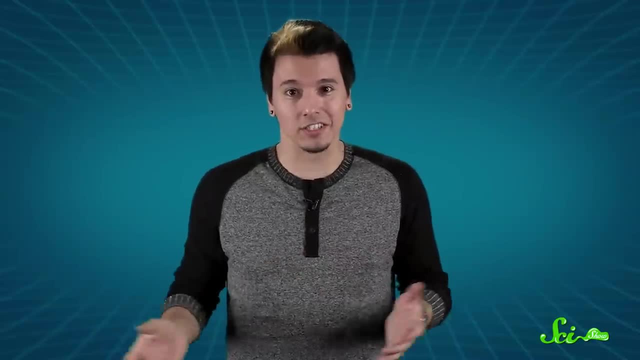 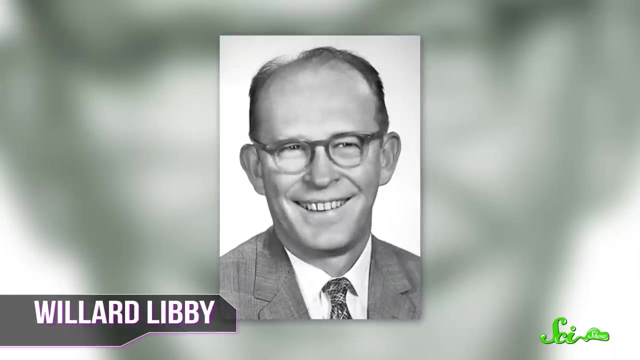 all you have to do is measure how much C-14 the dead thing has and do some calculations. Of course, figuring out how much C-14 a sample has turns out to be a little bit complicated. The first scientist to try it was American chemist Willard Libby in the 1940s, who used 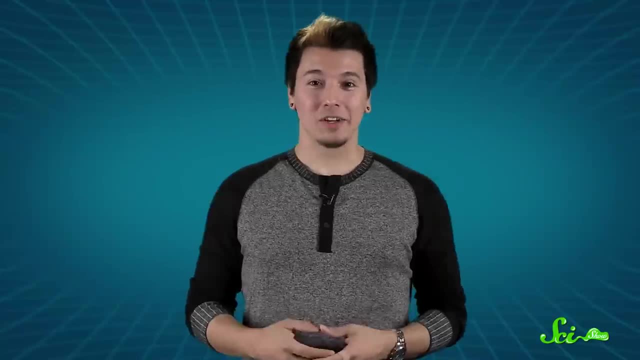 a Geiger counter to measure how many beta particles a sample spat out over time. He could then calculate the proportion of carbon-14 and figure out the age of the sample. Libby ended up winning the Nobel Prize in Chemistry for 50 years. 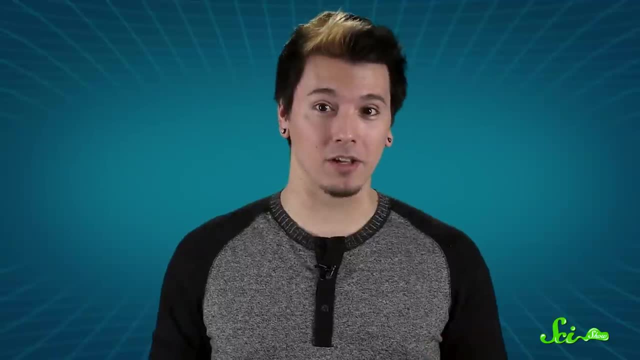 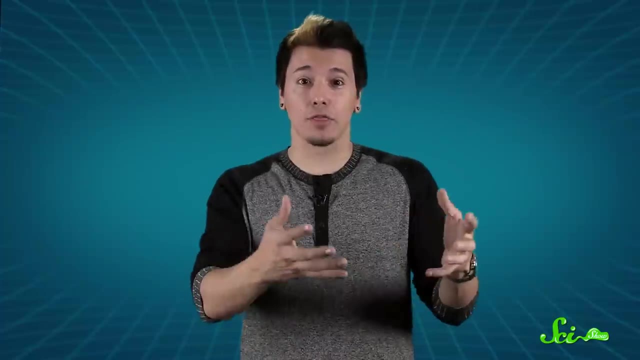 But since the late 1970s scientists have been using a better method called Accelerator Mass Spectrometry or AMS. In this rather long and expensive process, a sample is bombarded by ions, shot through a particle accelerator and finally separated by magnets to isolate individual carbon atoms. that can then be measured. AMS is a lot more accurate than the beta decay method, but its range is only about 50,000 years, because at that point there's so little C-14 left that we can't reliably detect it. 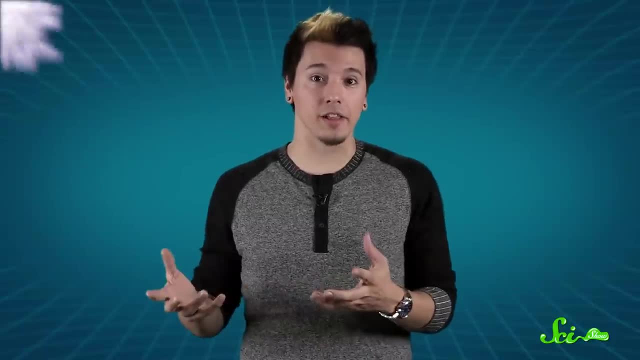 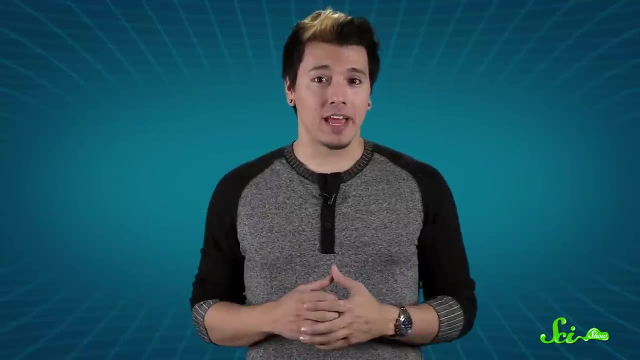 So to date, samples that are older than that like fossils. scientists track other elements like uranium or potassium, Which have half-lives in the millions of years. But there are still other problems. It turns out that the amount of C-14 in the atmosphere has changed occasionally over time. 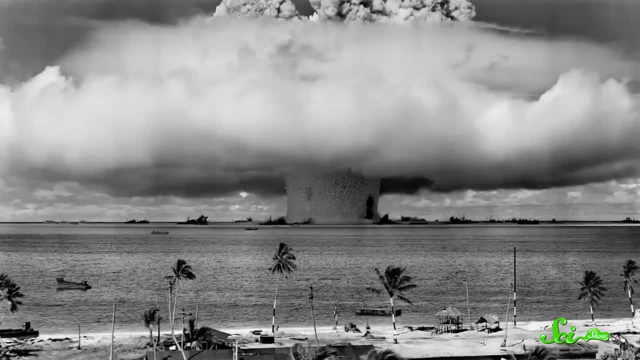 Several decades' worth of nuclear bomb tests in the 20th century, for example, managed to create a big spike in the amount of C-14 in the atmosphere, But at the same time, all the carbon being vaulted into our atmosphere by burning fossil. 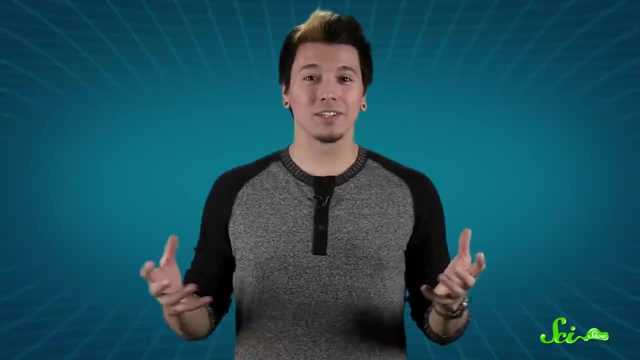 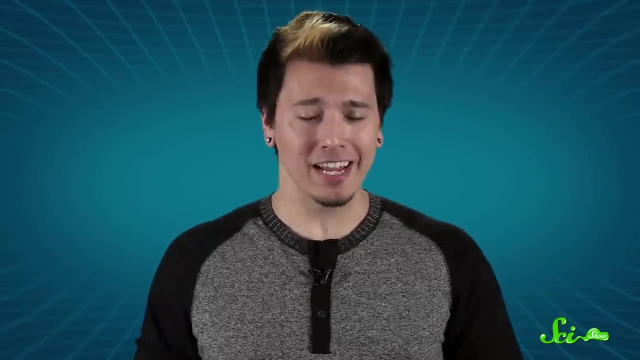 fuels may actually be diluting concentrations of the isotope. As a result, scientists often have to combine radiocarbon dating with other methods, like tree ring dating, to corroborate their findings. I mean, you probably already know this, but dating is hard.